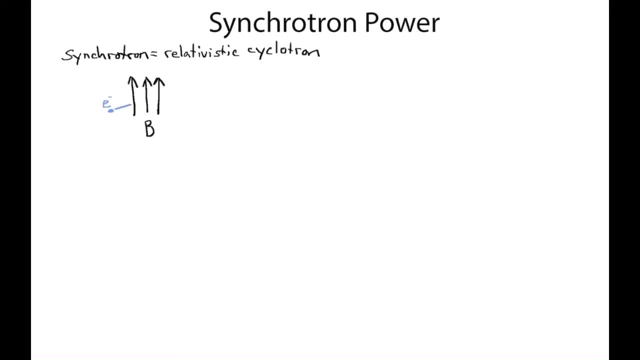 B in a charged particle, like an electron here, comes in at relativistic speeds and starts orbiting due to the force of the magnetic field interacting with the velocity of that electron. the acceleration of that electron generates emission which is radiated out from that electron over some beam. And these photons, these synchrotron photons, are what 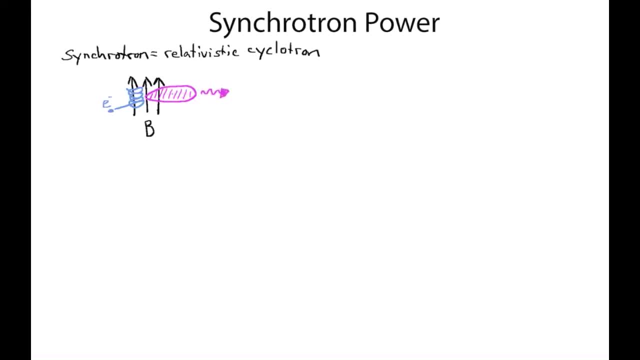 are carrying the power of the synchrotron radiation for us to observe Now. previously we had examined how, if I look at that same magnetic field, this time with the field lines going into the page here, and for an electron traveling around in a circular orbit here, 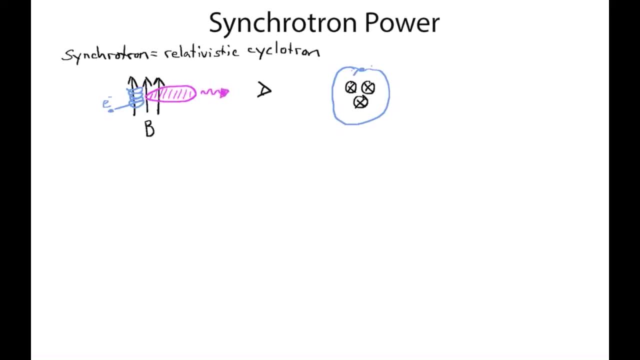 we derived that, even though in the electron's reference frame it thinks it's emitting cyclotron power, which has a characteristic symmetric pattern: forward and backward relative to the direction of the acceleration, which is down towards the center of this circle For synchrotron radiation, when this electron 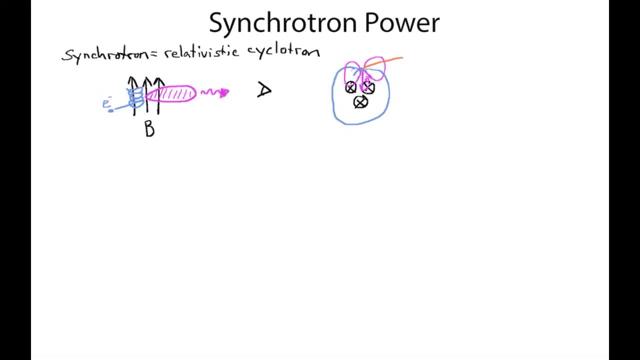 is moving at relativistic speeds, this radiation pattern becomes highly beamed in the forward direction, with very little power radiated in the backward direction and with a much narrower beam And, as a result of this being much narrower, an observer observing synchrotron emission receives photons for a shorter period. 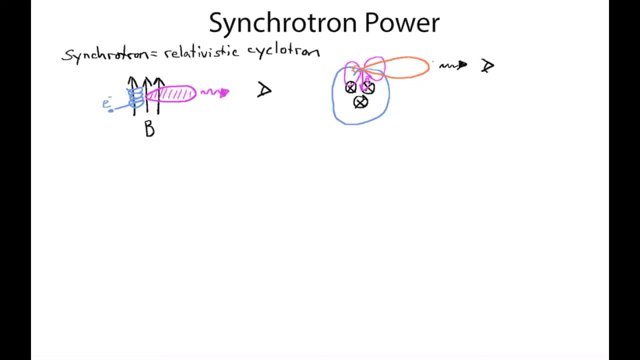 of time, which is only the period of time when this electron happens to be beamed toward the observer here And, as a result, synchrotron emission, instead of happening at a characteristic cyclotron frequency: omega cyclotron, which is the charge of the electron, times the strength. 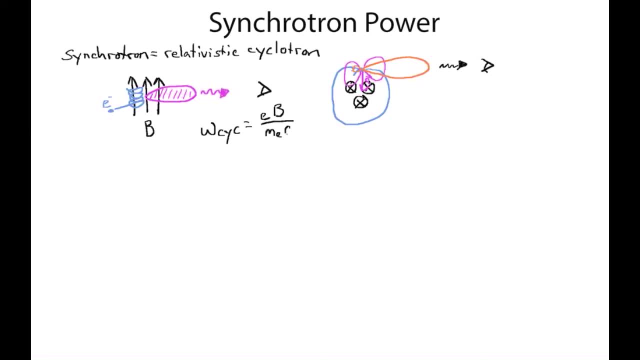 of the magnetic field over the mass of the electron times. the speed of light. Synchrotron emission arrives at a variety of frequencies up to a characteristic cutoff, which we'll call omega-sync cutoff, that we take to be 3 halves gamma squared omega cyclotron times sine alpha, where alpha was the angle that the electron's 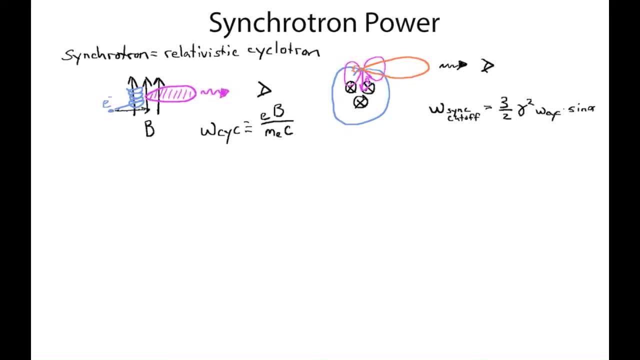 velocity makes relative to being perpendicular to the magnetic field. So this angle right here is alpha, And gamma is the Lorentz factor, which is 1 over the square root of 1 minus the velocity over the speed of light squared. And because of this gamma factor, or gamma, 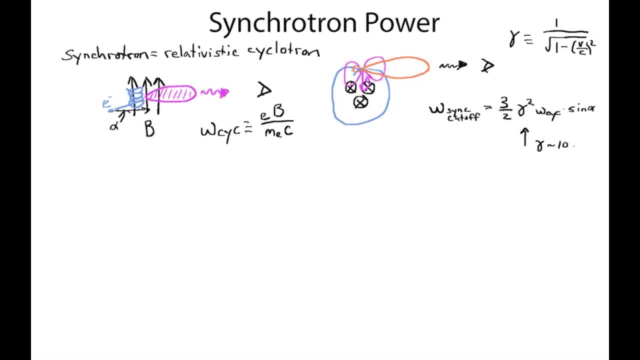 for highly relativistic electrons can be of order ten to one hundred. synchrotron emission is much harder than cyclotron emission, Which is to say it ranges up to much higher energies. So we're going to try to derive based on the 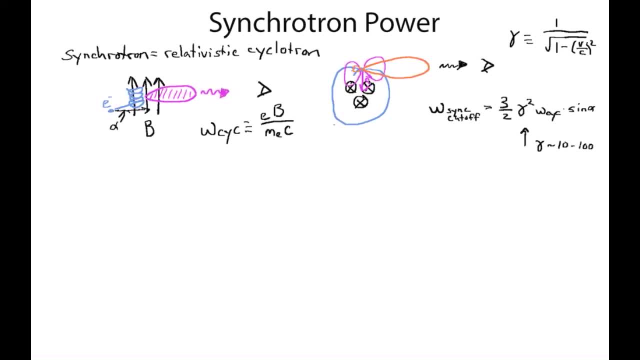 potential increase here in this, given Fen המ�, who is left up in the association with energy of the photons that are emitted by this electron over the relevant time intervals? how much power is radiated off by the electron for synchrotron emission? 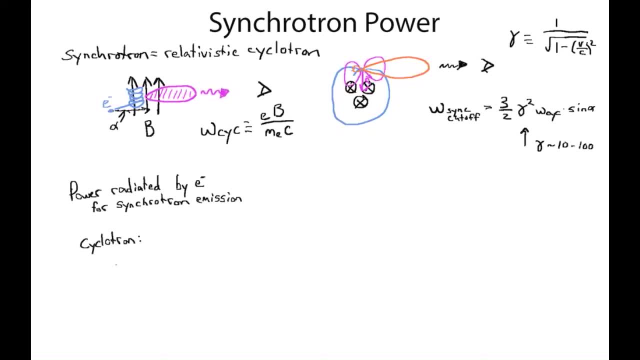 So first we'll begin with the cyclotron case. So a result we derived for the cyclotron case and is quite general for an accelerated electron, is called Lamer's formula, which says that the power radiated is equal to 2 thirds the charge squared times the acceleration squared over the speed of light cubed. 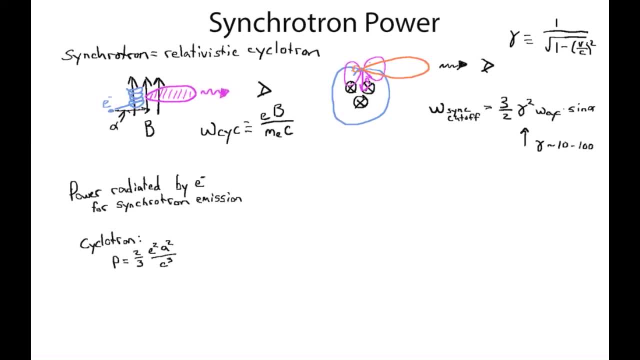 Now, in the electron's rest frame, that is, when we're moving along with the electron, it feels that it's undergoing an acceleration, but it doesn't know that it's moving relativistically. So in the electron's rest frame it thinks it's emitting according to cyclotron emission. 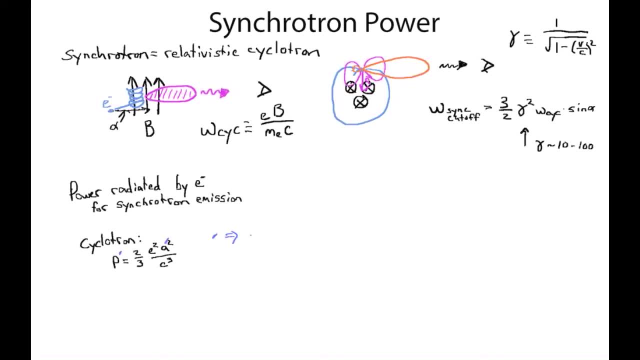 So I'm going to put a little prime here to indicate that we're in the electron's rest frame And the key to deriving this for synchrotron emission is to move into the last frame. This is the laboratory frame where this electron is moving relativistically. 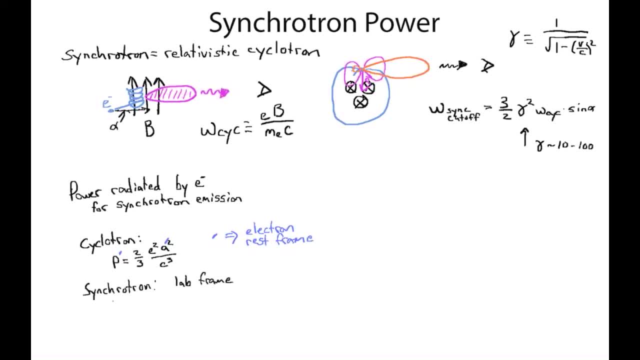 So for synchrotron emission we want to be in the lab frame, And it turns out this isn't so hard because power is a Lorentz invariant, which means that under Lorentz transformations power is unchanged. Everybody can agree what the power radiated is. 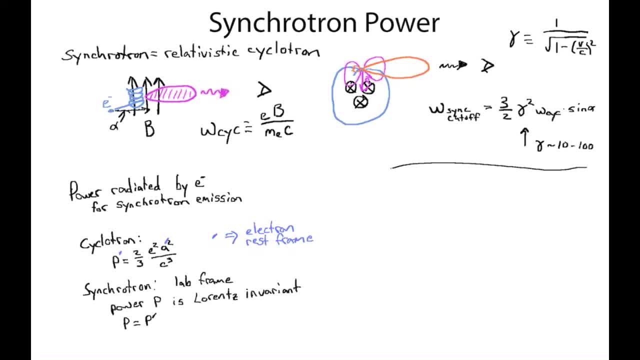 So in the lab frame p is just equal to p prime. And as a little aside here, we'll show that power is a Lorentz invariant. So power is the change in energy per time And we're going to use a derivative. 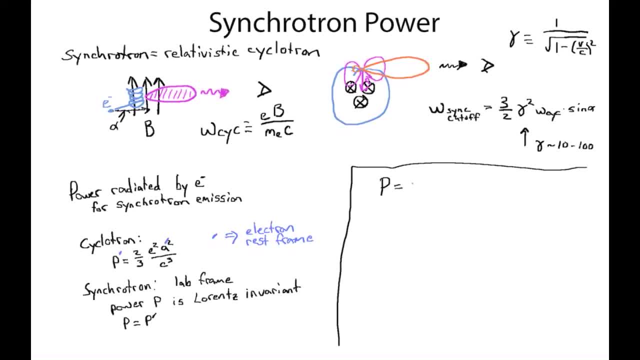 We're going to use a different letter for energy rather than e, because we're going to start using e to mean electric field in just a second. So we'll use w instead. Power is the change in w with time. Now, in special relativity, energy combines with momentum in a four vector. 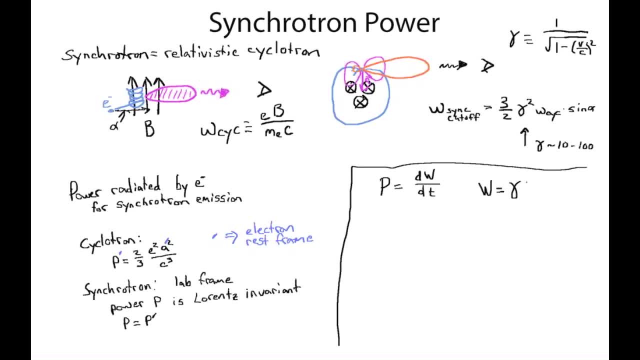 So that under a Lorentz transformation, energy is given by gamma times the energy in the prime frame, minus the velocity, v times the momentum, p, And without loss of generalization we get p prime. So in terms of generality we'll just assume that our velocity is moving in the x direction. 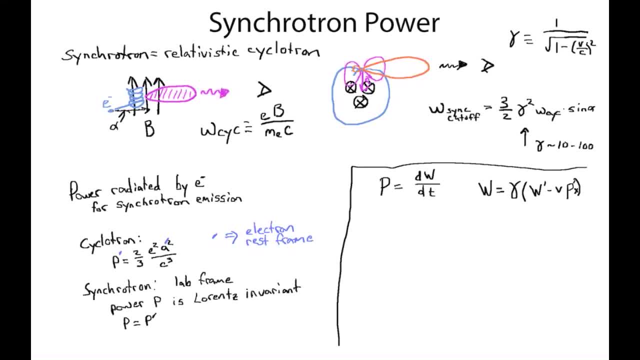 So we'll put a little piece of x for the momentum in the x direction, And this is also in the primed frame. And similarly time undergoes a Lorentz transformation that combines spatial and temporal coordinates in a four vector, So that t is equal to gamma times, t prime minus v, x prime over c squared. 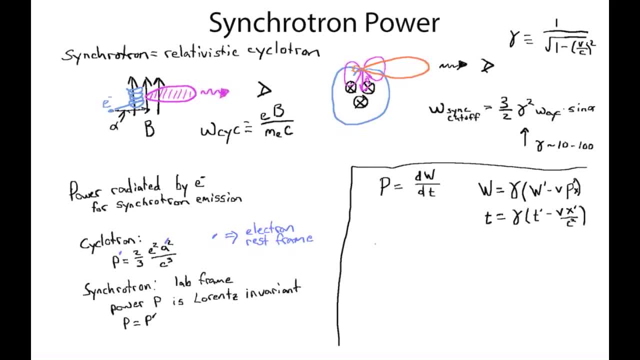 So we can see in the prime frame which will take to be the electrons rest frame, that frame, P prime, the power is dW prime, dt prime, And in the electron's rest frame there is no momentum and our x coordinate isn't going to change. dW prime, dt prime is in fact. 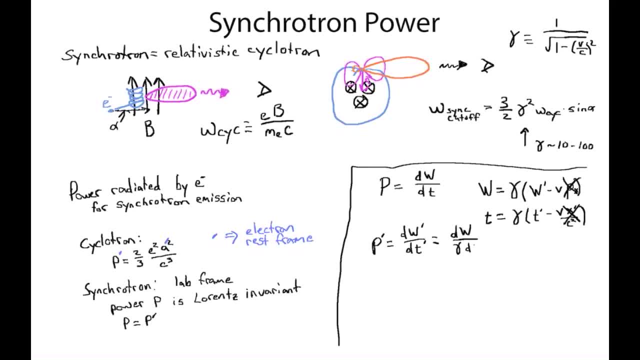 dW over gamma, divided by dt over gamma, And the gammas cancel out, and so we're left with P. prime is equal to P. So, given that power is a Lorentz invariant, in order to calculate synchrotron emission in the lab frame, all we have to do is calculate the power radiated. 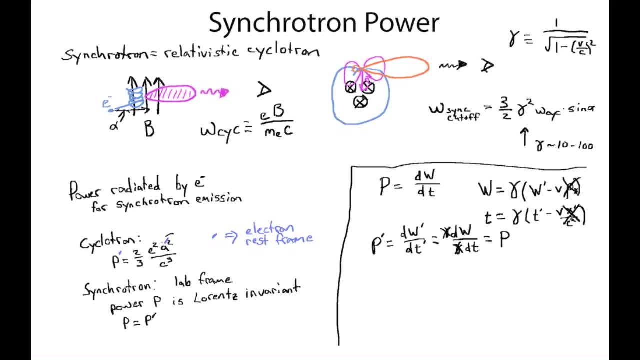 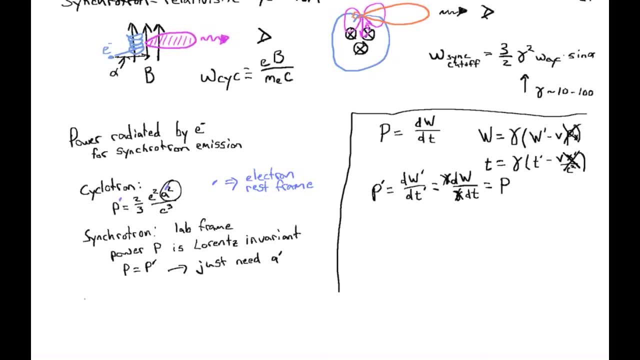 in the electron's frame, which really just means we need to figure out what A prime is And to get the acceleration in the electron's rest frame where velocity is zero. we need to determine what the electron perceives as the electric field, E, prime. And how do we? 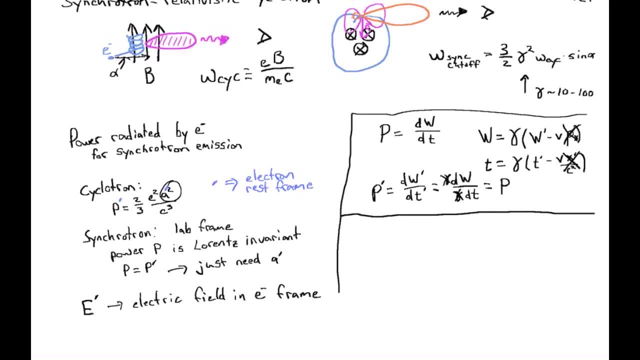 get an electric field in the electron's rest frame? Well, it just has to be a Lorentz shift B field. What the lab sees as this B field here must be Lorentz shifted into an electric field. In fact, the general case for how E and B fields transform under Lorentz transformations 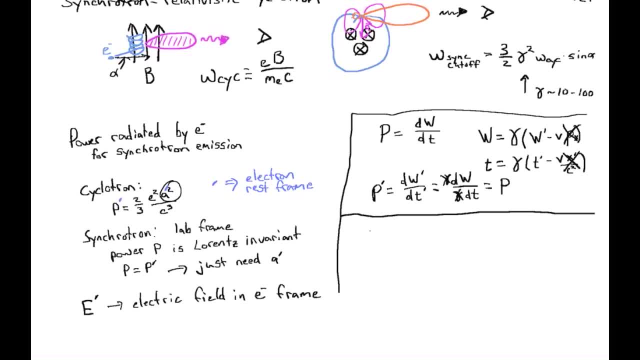 is that in the direction parallel to the velocity vector, the electric field in the prime frame is just equal to the electric field in the lab frame, And similarly the magnetic field parallel to the direction of the velocity is unchanged, Unchanged, Unchanged, Unchanged. 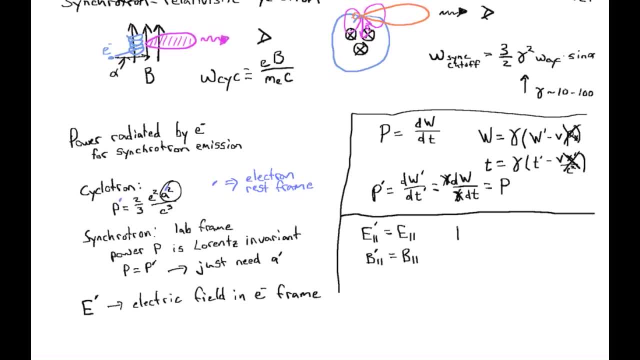 Under Lorentz transformation. But in the perpendicular direction the E field in the primed frame is equal to gamma times E perpendicular in the rest frame plus V over C crossed with the B field. There's no need to specify the B field in the perpendicular direction here. 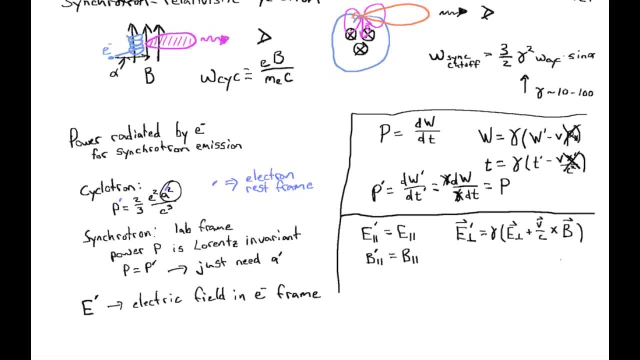 because the cross product here only extracts the component of the B field. that's perpendicular. And similarly the B field in the primed frame is equal to gamma times the B field in the lab frame minus V over C. So now we apply this to our specific case. here In the lab frame we have no electric. 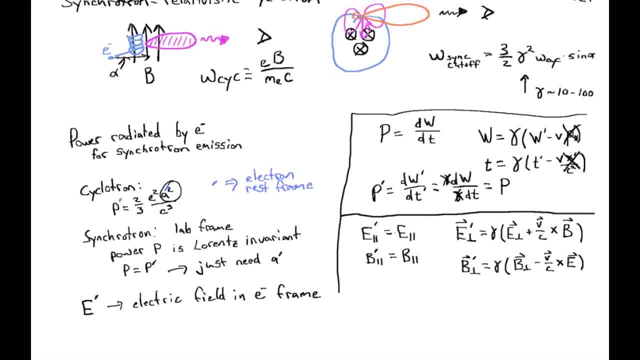 field and we're ignoring any interaction of the electron with its own electric field, as we have in all of our synchrotron derivations. So we can ignore this. And we're also not interested in any B fields in the electrons frame because the electron isn't moving. So 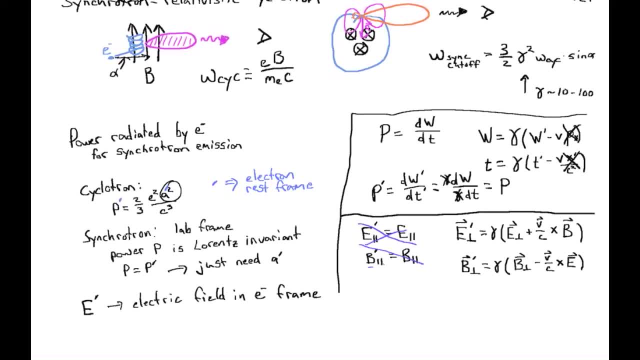 the B field can't be responsible for an acceleration. So we can ignore these And we're left with this term here, where in the lab frame we still don't have an electric field. So in the end the electric field in the electron's rest frame is given by gamma times. V over C crossed. 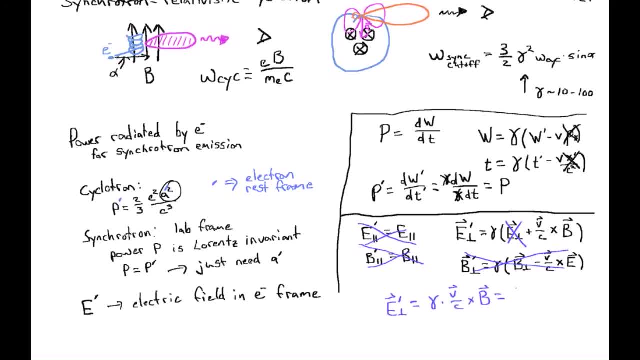 with the B field that we see in the lab frame And for the way we've constructed this problem. that's just gamma times B, the magnitude of the magnetic field, and then the component of the velocity that is perpendicular to the B field. 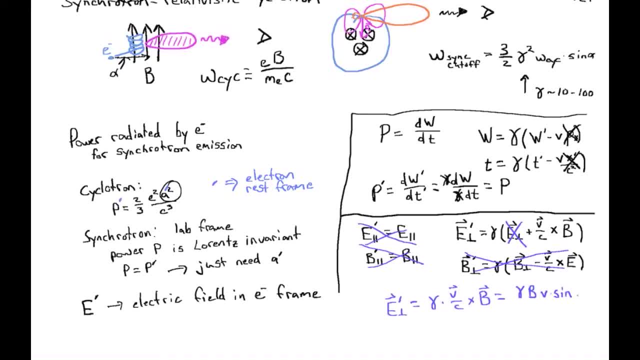 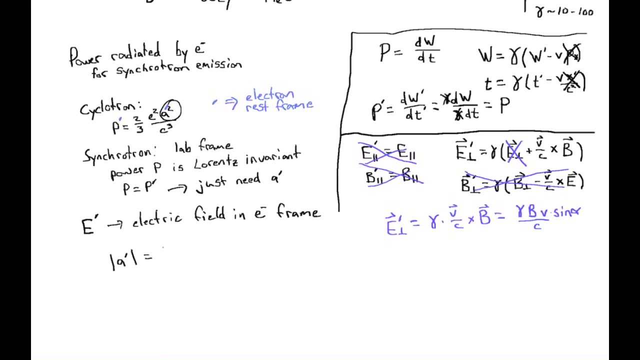 It's just V times sine of alpha. Alpha, you remember, was that angle to which the velocity of the electron is inclined relative to the B field over C. So that just means that the magnitude of the acceleration over here A prime is equal to E charge of the electron. 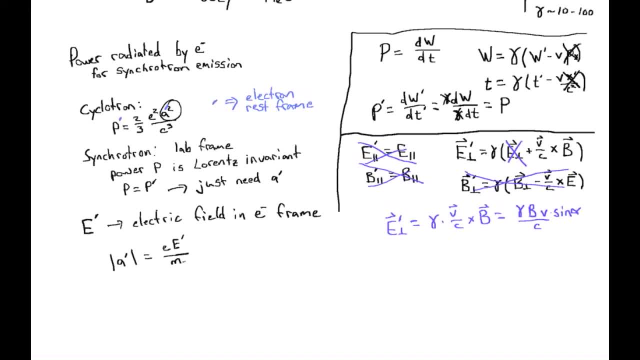 times E prime the electric field over the mass of the electron, which is equal to E B over MEC times gamma, V, sine alpha. And that means that the power radiated in the electron's frame P prime. if you just do the algebra out is 2 thirds E to the fourth gamma squared B squared, gamma squared V squared. 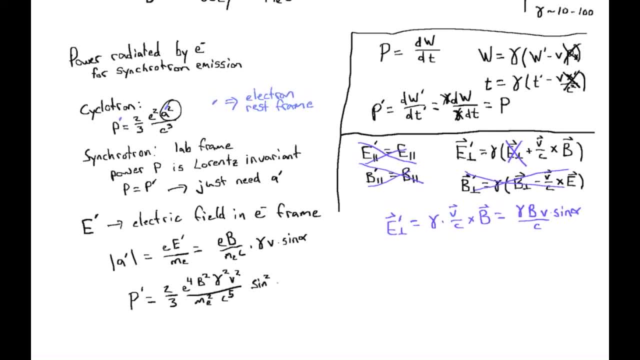 over ME squared C to the fifth sine squared of alpha, And recognizing that we're highly relativistic here, where we're taking the velocity of the electron to be very close to the speed of light and this power, as we discussed before in the electron's frame, is equal to the power radiated in the electron's frame P prime. 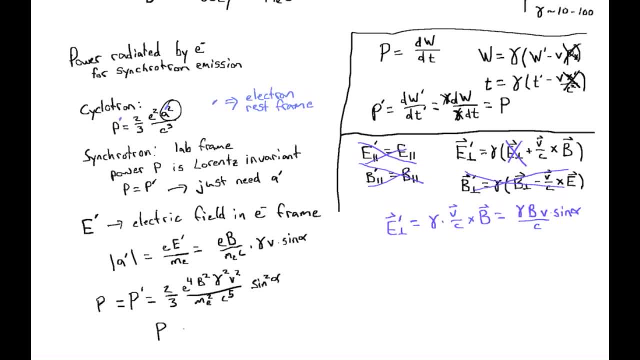 And that means that the power radiated in the electron's frame- P prime, if you just do the power radiated in the lab frame, So in the lab frame where this electron is traveling at a velocity that's very close to the speed of light, so much so that we'll just take V to be C, we get the power- is 2. 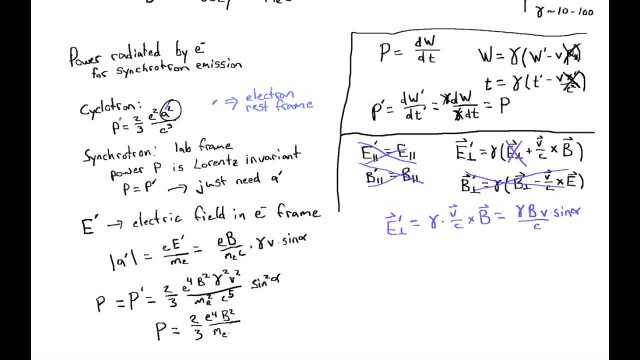 thirds, E to the fourth, B squared over ME, squared C, cubed times gamma squared sine, squared alpha. If you compare that to the cyclotron case, where the acceleration is given by E, V over C times the magnetic field, B Divided by the mass of the electron. 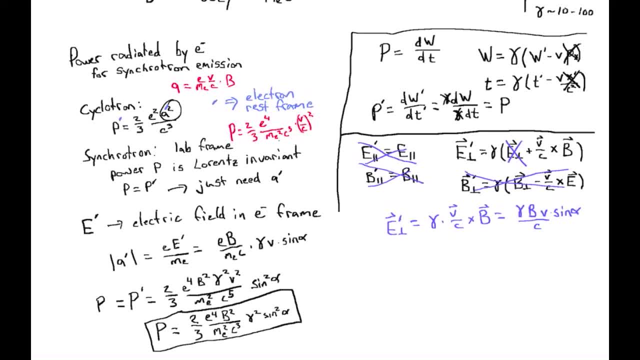 So that the power ends up being 2 thirds E to the fourth over ME squared C cubed times V over C quantity squared. Compare the cyclotron emission to the synchrotron emission. you'll see that synchrotron radiates power much faster by a factor of gamma squared and by a factor of C over V squared. 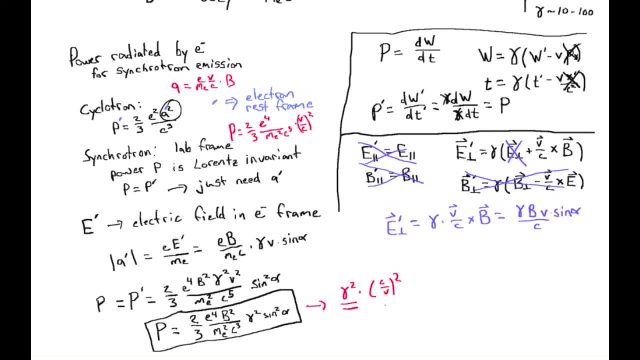 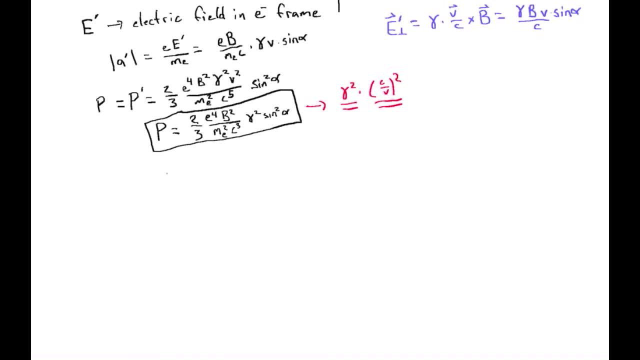 So synchrotron radiation radiates so much more power, both because it's got a Lorentz transformation here, A gamma squared, And because it's just going so much faster, so that B is much closer to C. And one more thing that's worth noting is we can write this power radiated in a different 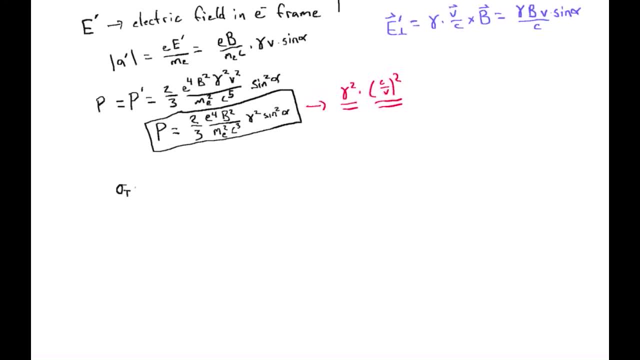 way, If you remember the Thompson cross section, sigma T, which was 8 pi, over 3 times the quantity E squared over ME, C squared, Whole thing squared, Then you can see that there's a sigma T in here. We could write that the power radiated by synchrotron emission is equal to 2 sigma T. 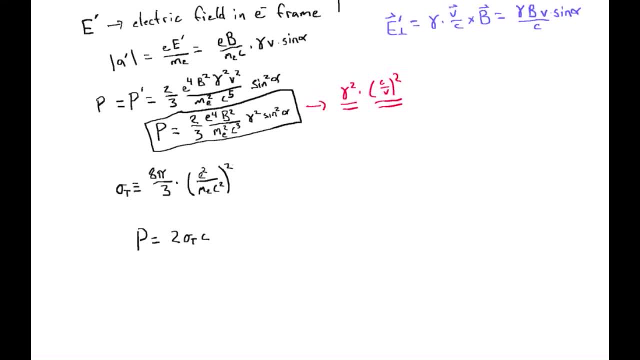 times C. We pick up the sigma T here. We pick up another factor of C here, because we have a C to the fourth in the Thompson cross section, but only a C cubed in our expression for the power radiated by synchrotron radiation. 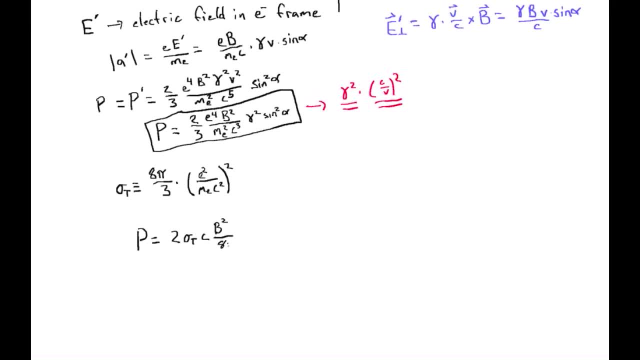 And then we end up with a B squared over 8 pi. This is where our 8 pi from the Thompson cross section gets divided back out: Gamma squared sine squared alpha. And this quantity- here the magnetic field- squared over 8 pi, is just the energy density. 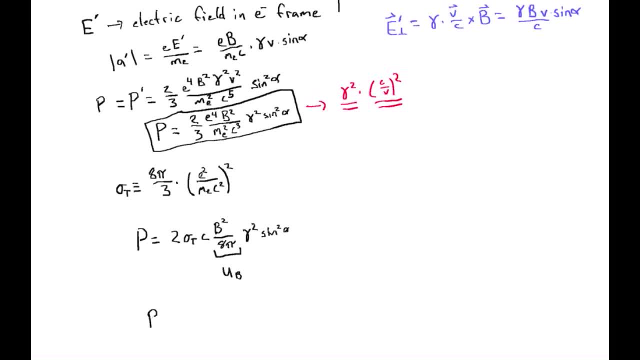 in the magnetic field: U sub B. So another expression for the power radiated by synchrotron radiation. So the power radiated by an electron through synchrotron emission is 2 times the Thompson cross section times, the speed of light times the energy density in the magnetic field times. 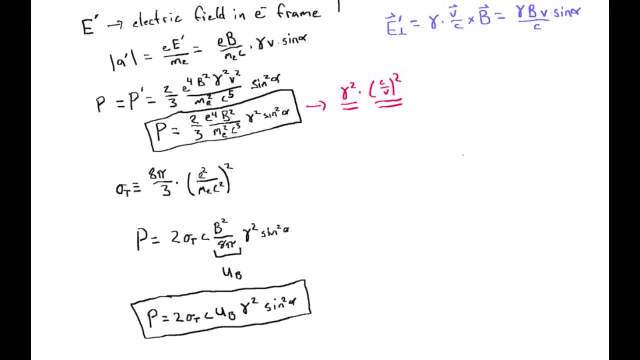 gamma, squared sine, squared alpha. So, given these two equivalent ways for expressing the power radiated by this electron, we're going to estimate a couple of time scales. One time scale is the lifetime of this electron emitting synchrotron emission. So how long can its electron emit synchrotron emission? 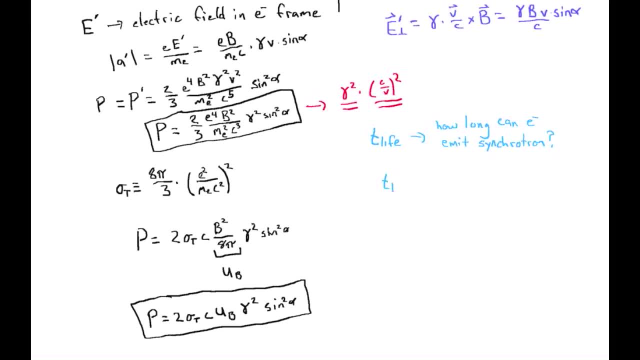 How long can its electron emit synchrotron emission? How long can its electron emit synchrotron emission? So this is thelarınstateumonization изб 2p, and it has to be something like the total energy of that electron which we will take to be gamma mec squared. 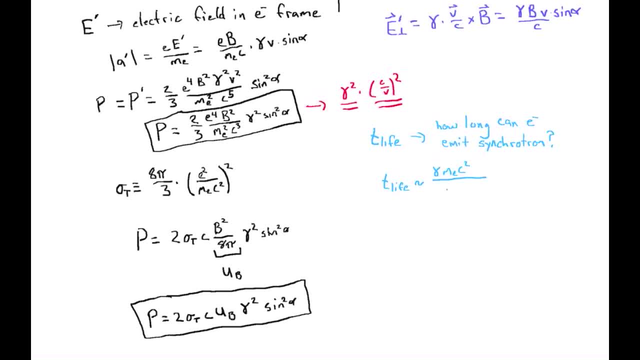 Divide it by the rate at which it is losing that energy, so the power, And we will ignore our factors of order. YU дан UWander tthattn- unity here. so we will ignore our sine squared alpha and our two thirds. and this is just dividing by e to the 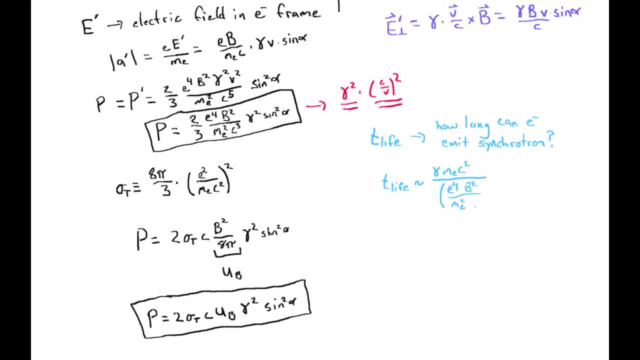 fourth b, squared over me. squared C: cubed times: gamma cubed restrict it to zero times. that is negative And that comes out to me the anfri. what does this mean, guys? negativeCOM spoke me Lee Lee, lee word. connectivec equals negativeSee2 toughty target Add. we better calculate the power. 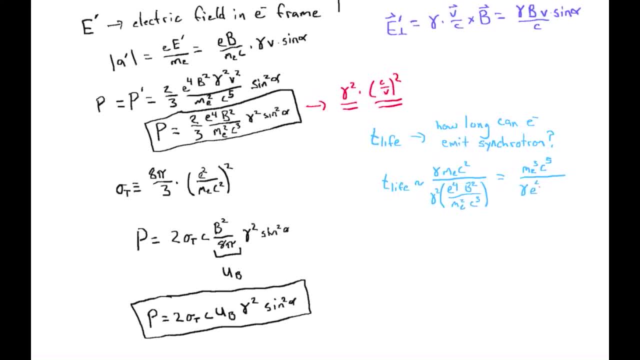 over adapting neighbors to the P. i sub at jp times gamma squared c to the fifth over gamma e to the fourth, b squared. So something to notice here is: the faster the electron is going, the more quickly it decays And of course the stronger. 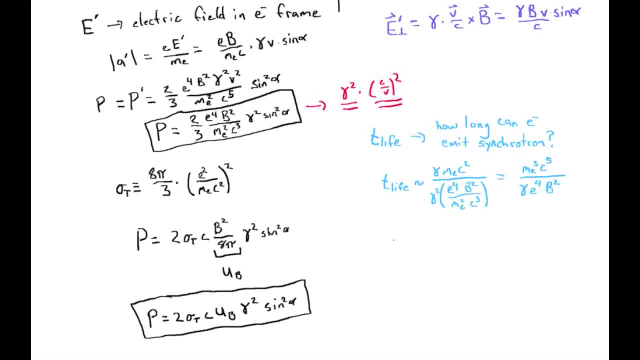 the magnetic field, the shorter it lives as well. We can compare this lifetime to say the time it takes to make an orbit which is of order 1 over our orbital frequency, which we derived previously to be e, b, over gamma, m, e, c. So 1 over that will be gamma. 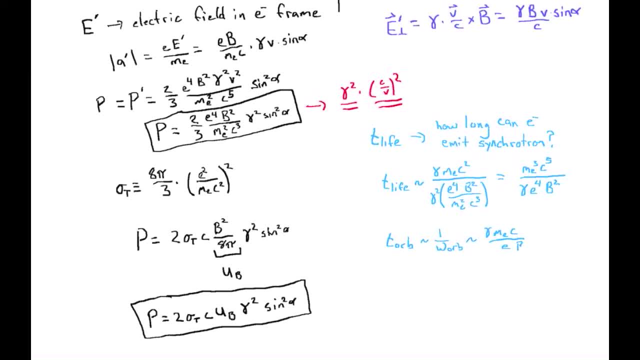 m e c over e b. An interesting question is: what would it take for the lifetime to be of order 1 orbit? If you work out the algebra you get that gamma squared b should be of order c to the fourth m e squared over e cubed. So you plug in 3 e 10.. 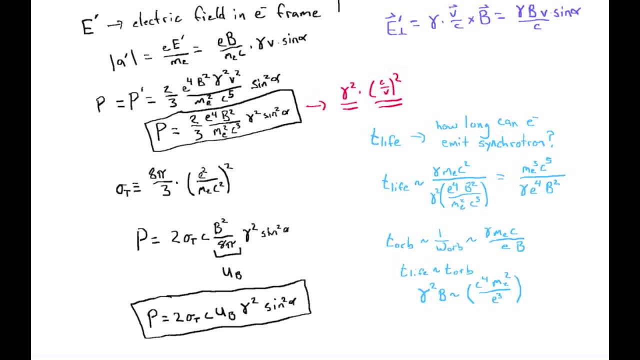 1 e minus 27 for the mass of the electron and 5 e minus 10 for the charge of the electron, all in CGS units and we end up that this should be something like 10 to the 16 in CGS. 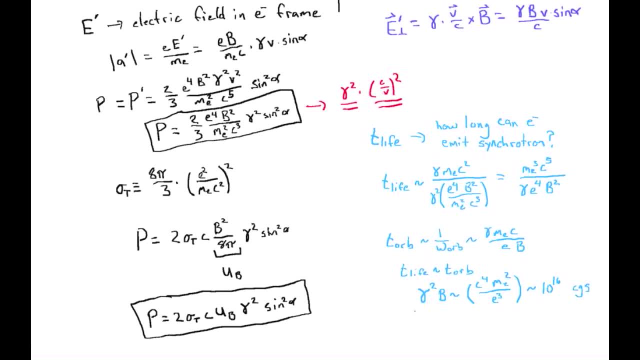 units for the magnetic field. So the answer here for values of gamma in the 10 to 100 range is a b field of order 10 to the 12 to 14 gauss, which is worth noting, is a very strong magnetic field. One more time. 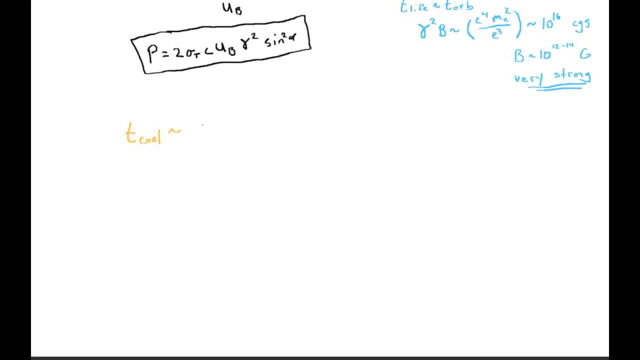 One more time scale we can look at is the cooling time, which we'll set up the same way as our lifetime calculation. It's the energy of the electron, but this time we'll put in our other expression for power, just to mix things up: 2 sigma, t times, c times. 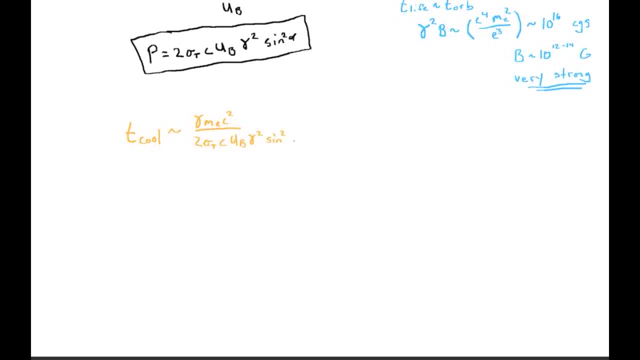 the magnetic field energy gamma squared sine squared alpha, And we can take sine squared alpha in an ensemble average to be 2 thirds averaging over a sphere. So we can plug in the values here. One of our factors of gamma cancels and you get that. the time scale is of order if you. 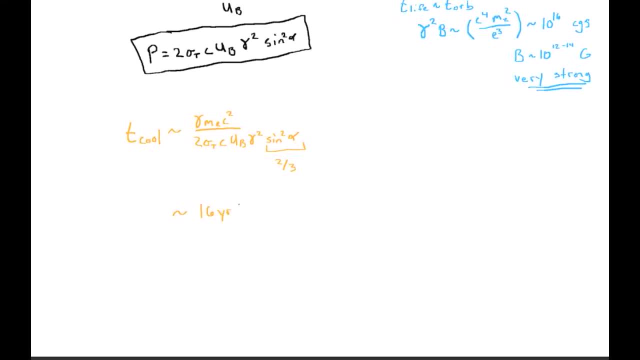 plug in a magnetic field of 1 gauss 16 years and that scales inversely with the square of the magnetic field strength, So 1 gauss over b squared, and it also scales as 1 over gamma here. Now let's do a couple real world reality checks here For something like a. 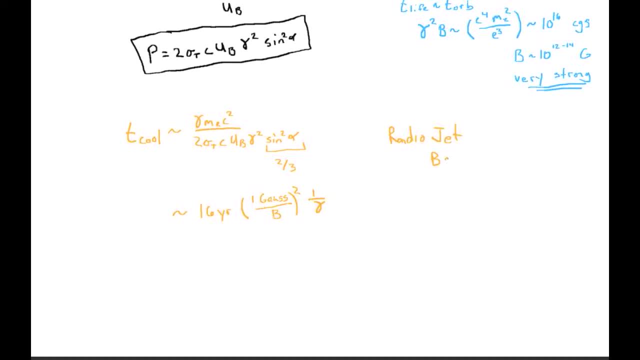 radio jet. where we can the magnetic field to be of order a milligauss and where gamma is actually really large like a thousand, we get that the cooling time is of order ten thousand years, which is roughly comparable to the dynamic time for 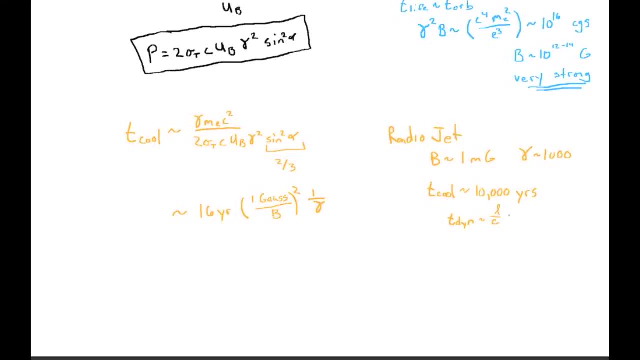 something moving at the speed of light to cross a length L of one of these jets, which is of order a kiloparsec. This works out to be about the same time scale, ten to the four years. You can also look at something like a supernova. 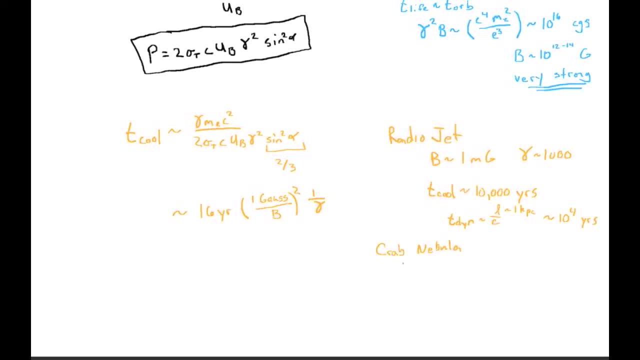 remnant like the Crab Nebula. Now, for the Crab Nebula, we'll do something a little different. We'll take the magnetic field to be of order a milligauss, but instead of assuming a gamma, we'll pick an energy of a photon that we're. 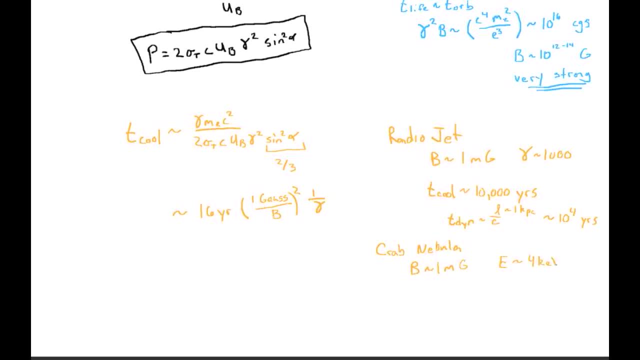 observing with something like a four kiloelectron volt photon. Now, via our expression for the critical synchrotron frequency, omega C, which was three halves gamma squared times the cyclotron frequency, and we'll ignore terms of order unity, like three halves and sine alpha. And if 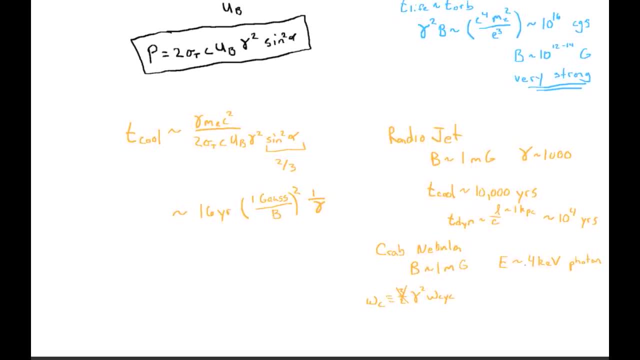 we just pretend that all of the photons that come to us at four keV were generated by electrons moving at this critical synchrotron frequency. then E, which is h-bar omega, we can take to be h-bar gamma, squared times, Eb for MEC, the cyclotron frequency, and using this we can solve for gamma and plug that. 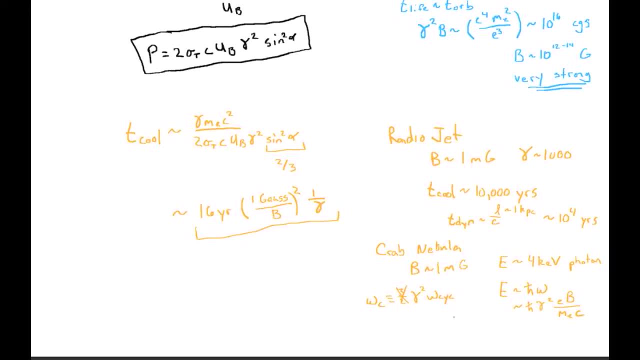 gamma into our expression for the cooling time here, along with our magnetic field, And we get that our cooling time is of order two years. That's interesting because we know the Crab Nebula was created about a thousand years ago, as observed by some Chinese astronomers. So this tells us that there. 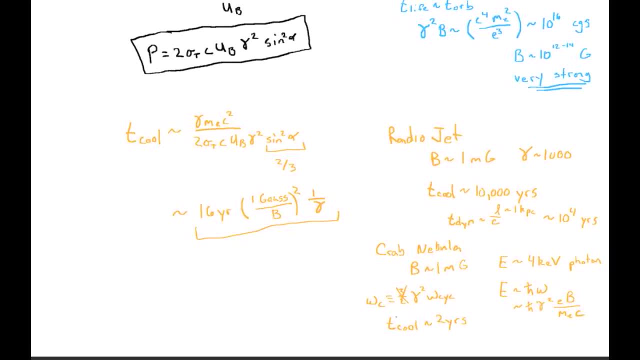 must be new sources of relativistic electrons in order to observe emission at four keV. Given that we do observe emission in this band- we get x-rays from the Crab Nebula- we know that there must be a new source of relativistic electrons and in 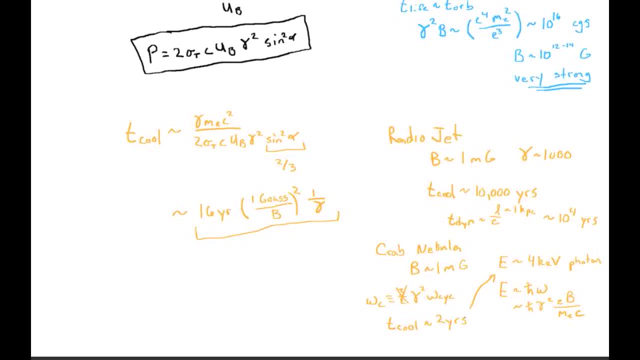 fact, those relativistic electrons are coming from the pulsar that's sitting in the middle of the nebula. So that's basically what I want to say about power radiation. for synchrotron emission, We have two expressions for the rate at which a relativistic electron in a magnetic field radiates: energy and our.